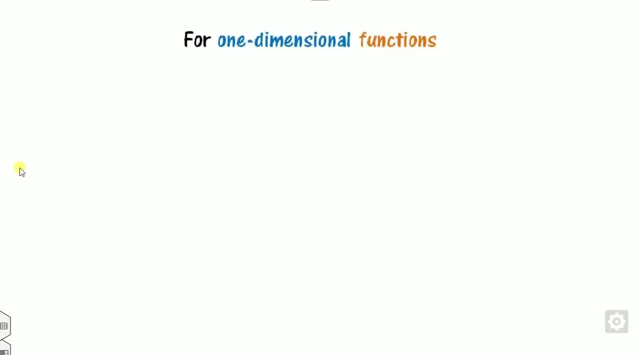 on my, either on this link or my playlist. So for this that. but the first method is that if your function is the first dimension is that there is a one dimension is problem- consists of only one variable, Then you can calculate the second derivative and you can check whether. 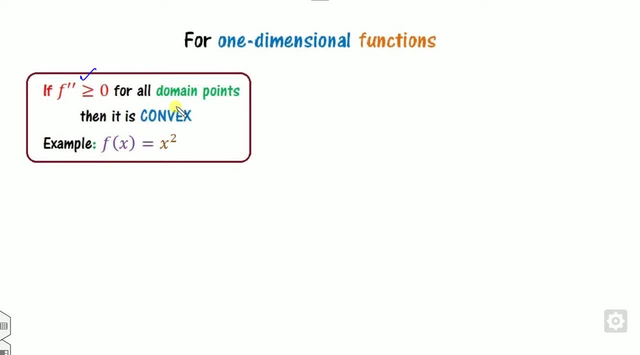 it is a convex. if it is greater than equal to zero, then it is a convex, otherwise concave. You can see if you, if you calculate the second derivative of this, this is two and which is a greater than zero For all the values of the x. so it means this is a convex. Similarly, if the function is: 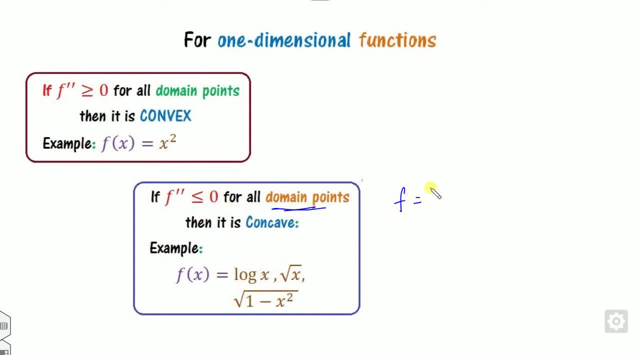 my less than equal to zero for all the domains. look at that: if I just take the function as a log of x, what is the first derivative is 1 by x. what is the second derivative is minus 2 by- sorry, minus 1 by x square, and this is less than zero for all x. Similarly, if you 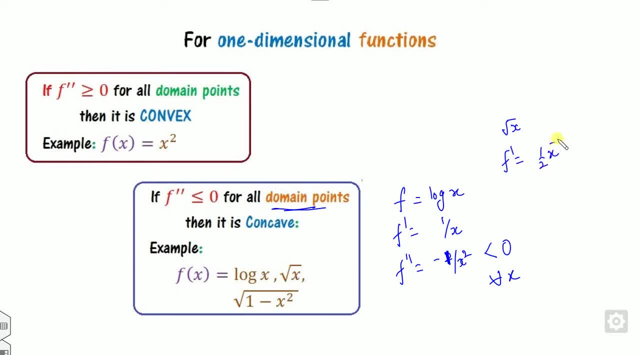 take the function as a root of x, then what's the first derivative is 1 by x, raised to power, minus 3 by t, 3 by 2.. Similarly, if the function which is neither the convex or nor concave, we call when, when the function second derivative is less than or greater than zero. look at that. if you take 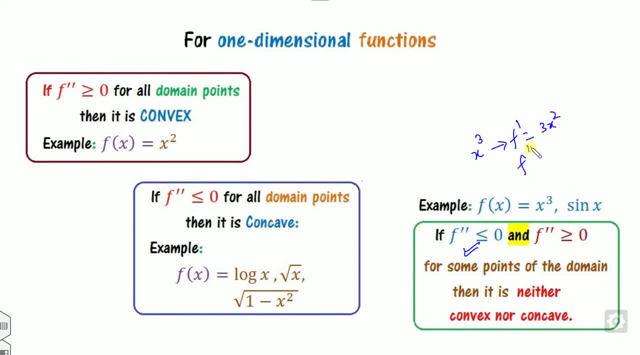 x cube. then what's the first derivative? is my 3 x square. what is the second derivative? is my 6 x. so it can be greater than zero. it can be less than zero, depending upon the value of x. Similarly, if you take the sine of x, what is the derivative of the first sine x? 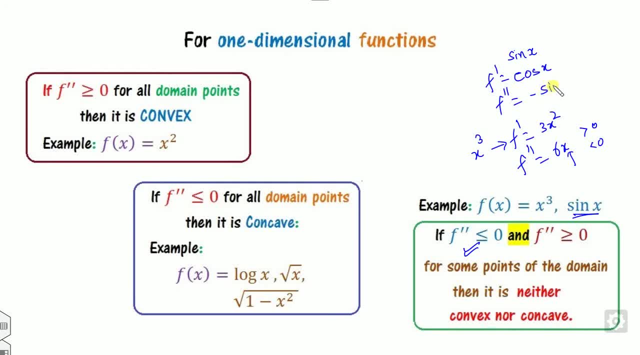 is x, and what is the second derivative is minus of sine x. so definitely minus of sine x. it can be greater than zero or less than zero, depending upon the quadrant where the x values lies. so therefore it can be neither be a convex nor be a concave. 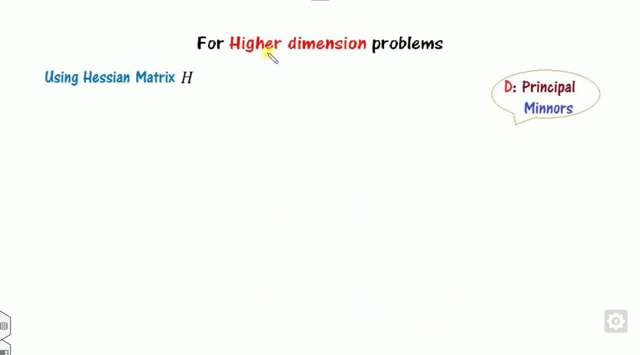 So this is the first method. you can check with the help of the one dimension. on the other hand, if you have the two dimension, then we will utilize the Hessian matrix. that is the last lecture where we can calculate the principal minus. If my Hessian matrix 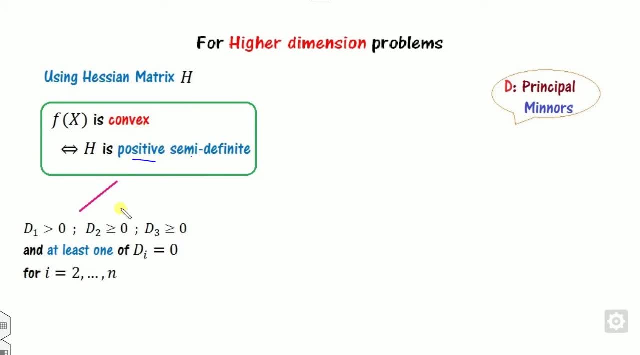 The Hessian matrix, the positive semi definite, then it is a convex. what is the meaning of the positive semi definite is all the principal minus are greater than zero and since, due to this semi, at least one of the principal minor is a zero, then it is called as the convex. 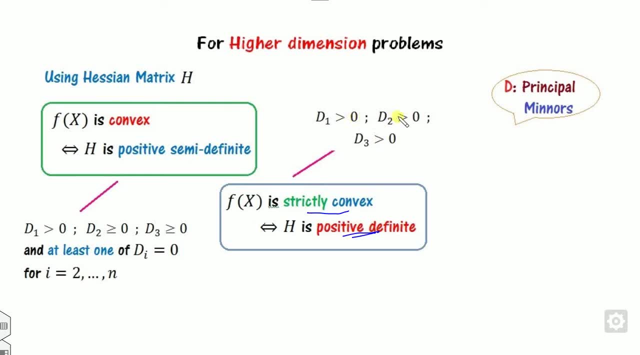 on the other hand, when it's said to be the strictly convex it. if it is a, all the principal minus are strictly greater than zero. Conversely, if I say, when the function is said to be concave, when minus of the f of x is convex. 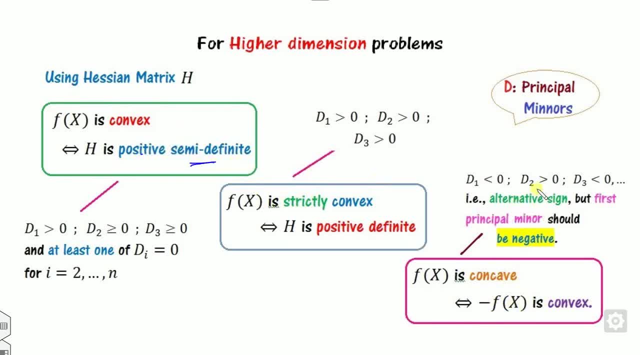 Or you can say When- When it is a negative semi definite. what is the meaning of the negative semi definite is they are of the alternating sign, but the first one should be a less than zero. Another one is that you can utilize this. with the help of the definition, you can say this: 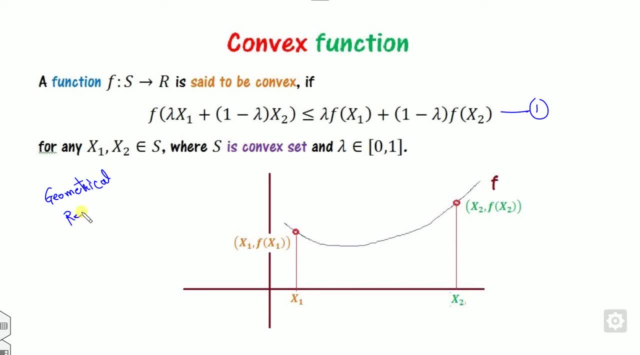 is the geometrical representation of. this is a geometrical representation of the convex set. what is the meaning is that you can draw the any function like, say, if you have x square, you can draw the function like this way- sorry, it's a horizon- if you have the function of, 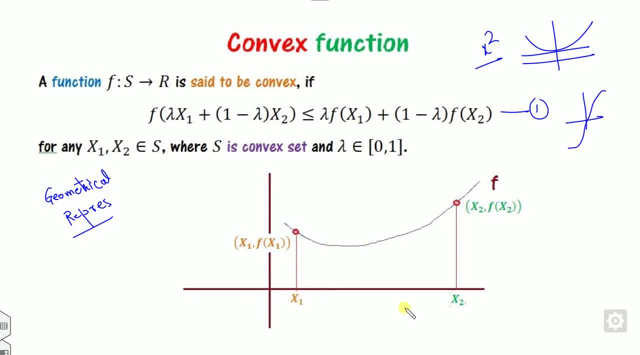 the x cube you can draw like this way, and so on. So take any two point in the domain x1 and x2, and these are the points of the x1 and so on. So look at that. what is that? this is nothing but the clc. this is the convex linear combination. 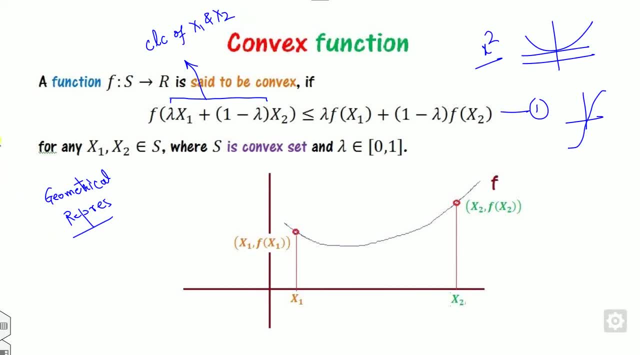 of the x1 and x2. so look at that in the graphically. what is the convex linear combination of x1 and x2? this one is there. what is the meaning of the f of x1? this is my f of x1, this is my f of x2. and what is that lambda times of this lambda, one minus of it means this is: 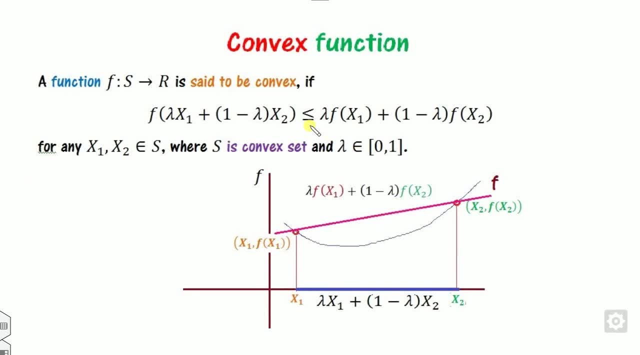 nothing but the convex linear combination of this. Now, according to this figure, what is that f of t convex linear combination? these are the f. so if you take at point, the value is here. if you take at point, the value is here and so on. So all those points which are lies on this below portion. so this is called as my function. 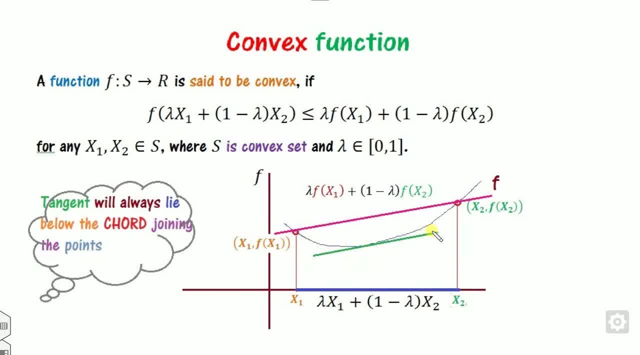 at the here. so, according to this definition, the tangent at this point, the all those points which are here, which are lies below to the code: Okay function is set to be convex. Otherwise, the function is set to be concave. So if your 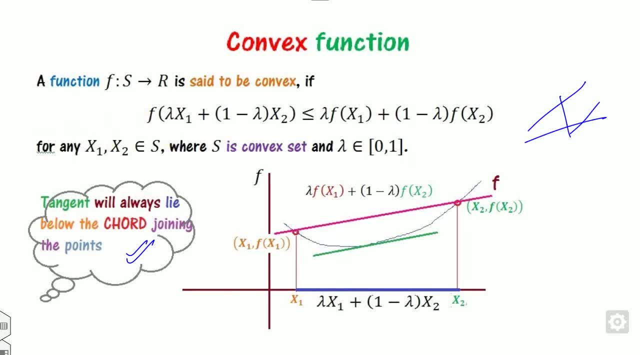 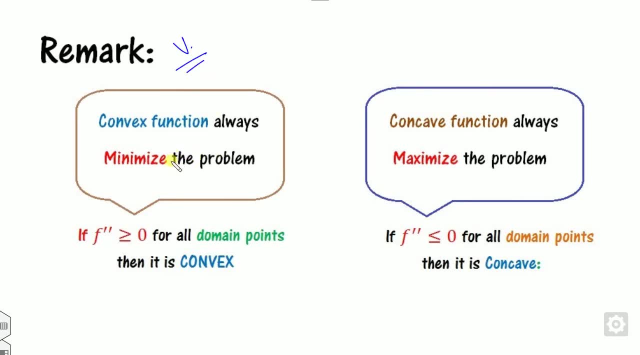 tangent is above and the code is below, then your function is concave. Now it's a very important remark for you. If you have the function f of x and you want to check whether it's a minimize the problem or maximize, you have to prove that if it is a convex, then it will always be minimized. 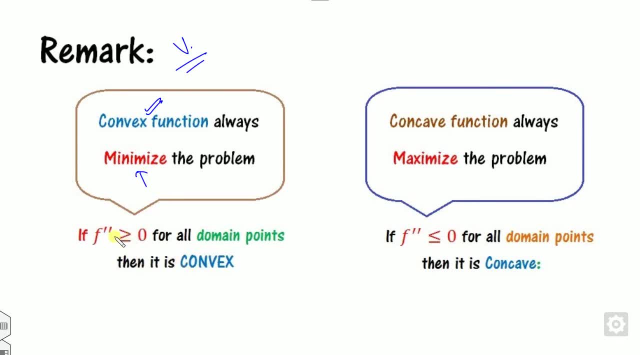 because you can see f double dash is greater than 0, then it's a convex. So what is the condition for that? This is always with a minimization. Similarly, if the function is concave, then it will always give you the maximize that. So, for example, look at that here- whether the function 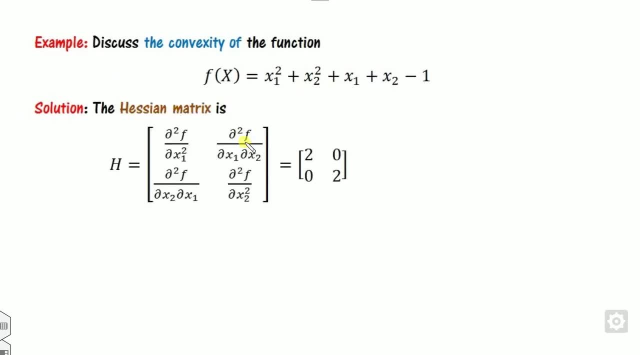 is minimization or the maximization, how you can check that. You have to draw the Hessian matrix because it's a two-dimension problem. So you can use the either the matrix minor, that is a principal. What is the principal minor of this? 2 and 4, both are the greater than 0. 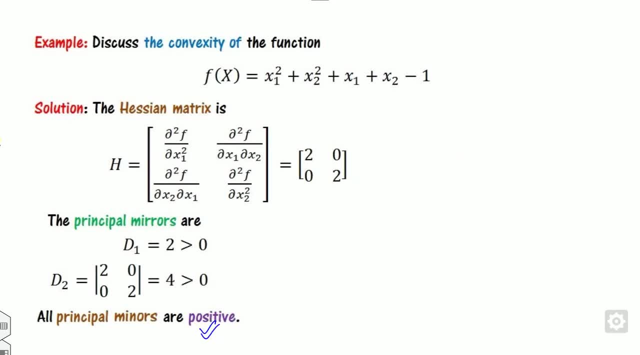 So it means it are positively definite. Else, you can also check with the help of the eigenvalues, Since both the eigenvalues are positive. so what is the meaning of that? It is a positive definite. So once it is a positive definite, since equality is not there, 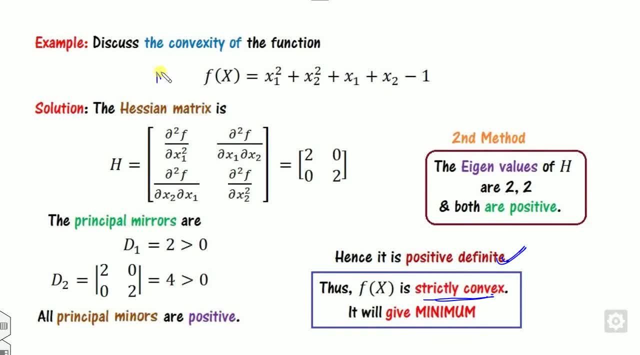 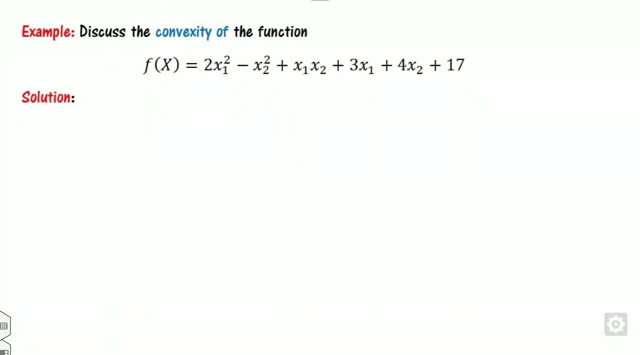 so it is a strictly convex. So once it is a convex, so it means this function will give you the minimization of the f of x. Similarly, if you take out the second function here, you can draw the Hessian matrix. that is the second derivative of this. 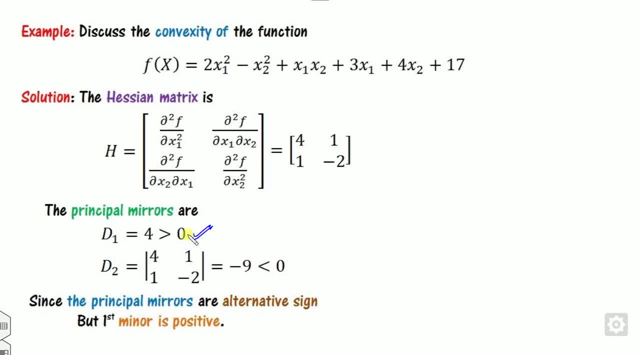 Once you are finding the matrix, principal, minor, you can see the first one is a positive, second one is a negative. there is an alternating sign, But the first one is a positive sign. So it means it is neither maximum nor a minimum. So therefore it will neither give a maximum value. 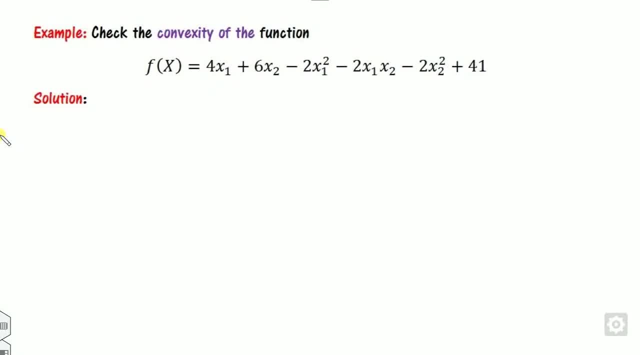 nor give a minimum value for the function. Look at one more example. If you have the function like this way, then how you can check that this? look at that. the Hessian matrix is this: If you draw the principal minor, you can see here, that is, they are the alternating sign. 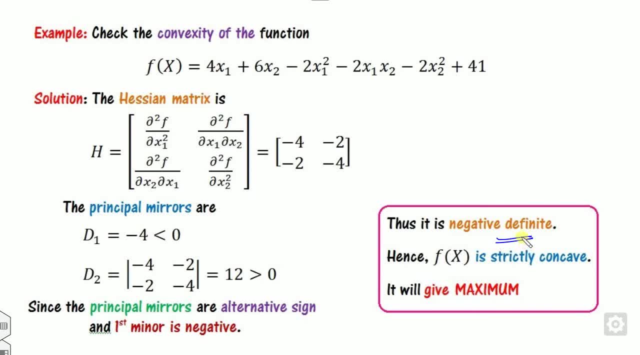 and the first one is a negative. So therefore it is a negative definite. So once it is a negative definite, it means it is a concave. So if it is concave, then it means it will give you the maximum value. This is the method. Again. 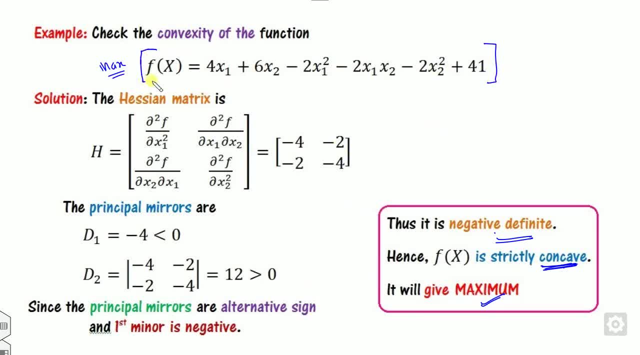 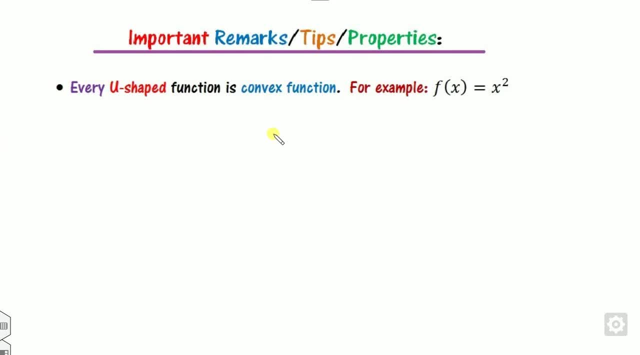 you can also think about without the solving this. you can think about the problem from here, where the function is convex or concave, how we can see important remarks is there? First one: if you draw the graph of the any function and if it is a u-shaped graph, 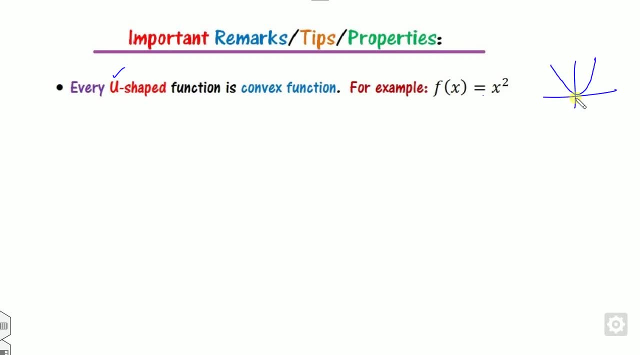 look like, say, x square. what is the function of the x square? is This So, since it is a u-shape, so every u-shape function is a convex function? Second point: is every function which is convex and concave- sorry, that function which is both? 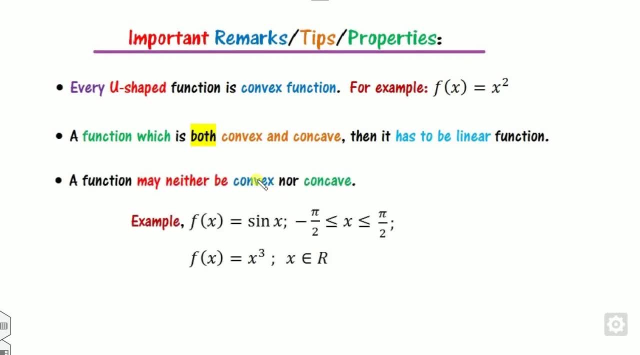 convex and concave is called as the linear function. A function which is neither the convex and nor concave is here. you can also check that, because the derivative is either greater than or this both at the same time. The domain of the convex function is the convex set. 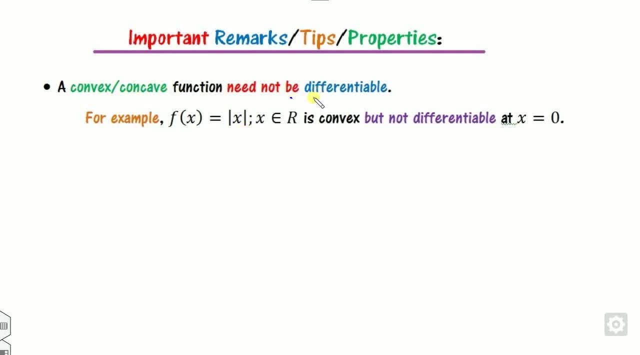 This is an important remark: The convex or concave function need not be differentiable. Look at that mode of x is always be a convex function because if you look at that, if you think about this, this is always be here. So if you apply the definition of the convex set, it is here but it is not differentiable at. 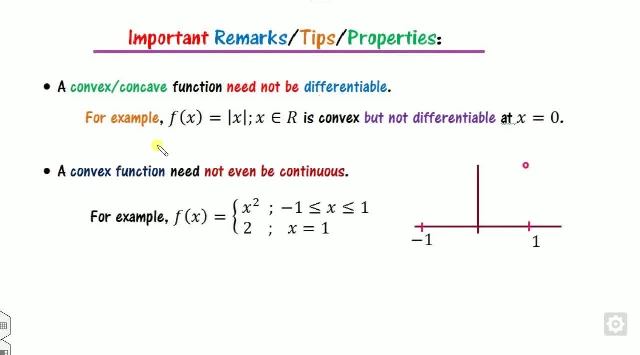 x is 0.. All of you know that mode f is not differentiable. Similarly, the convex function need not be even a continuous. If you draw the graph of this minus 1, so look at that. this is the graph of the x square. 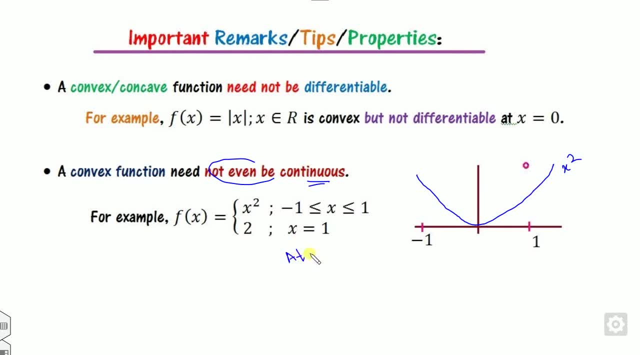 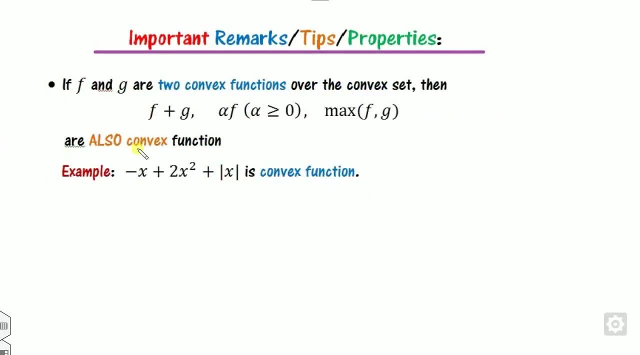 The convex function is always continuous in the interior of the domain. So if you consider this as open interval here- that is, the interior- then it is a continuous function. Most important remark is that the sum of the two convex function is a convex function: Scalar multiply of the two. 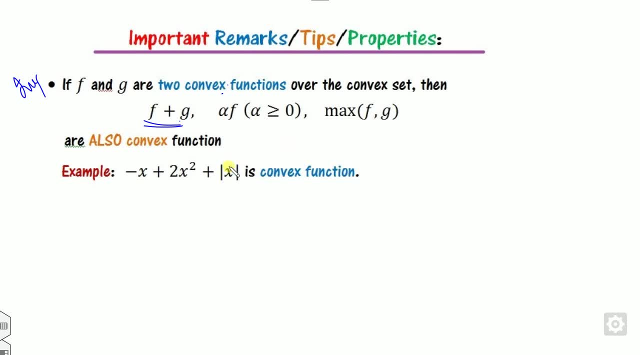 convex function is a convex function. Maximum of the two convex function is a convex function. Look at that. The one way is that you can check whether the f double dash is greater than 0 or not. then it is a convex. Otherwise, look at that: minus x, plus 2x square, plus mode of x. 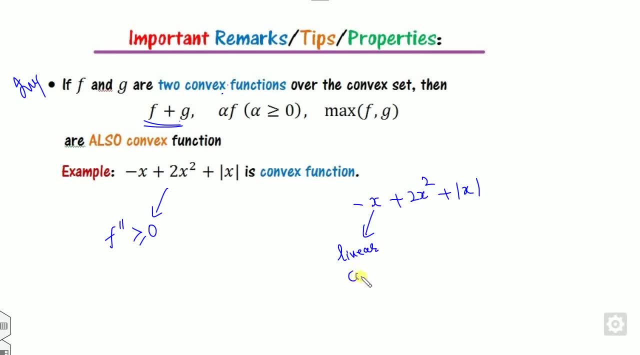 This is a linear function. Every linear function is a convex and concave, So it is a convex function. x square, the function you can check, simply you can check the double derivative of this. This is nothing but 4, which is greater than 0.. So it is a convex function. Mode of x. 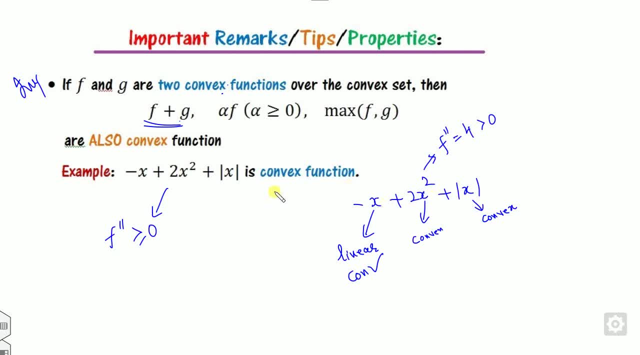 is always be a convex function. So it is again a convex function. So sum of the convex function is a convex function. Similarly, if you take as the concave function, then sum of the concave function is a concave Scalar multiply and look at that. here is the minimum of dampen. 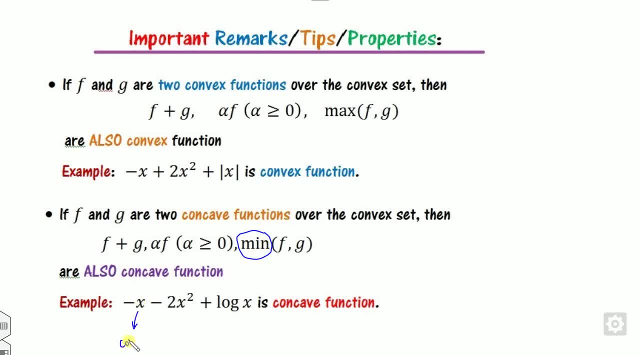 So look at that. This is a linear function. So every linear function is a convex and concave both. So it is a concave. Look at that. What is the derivative of this? What is the derivative of this? is minus 4 and it is a less than 0. So it is a concave. Look at the log x. What is the? 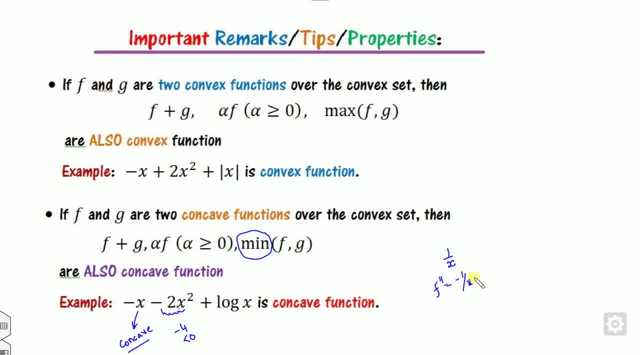 derivative of the log x is 1 by x. So what is the second derivative is Minus 1 by x, which is always less than 0. So it is a concave. So this is concave, this is concave, this is. 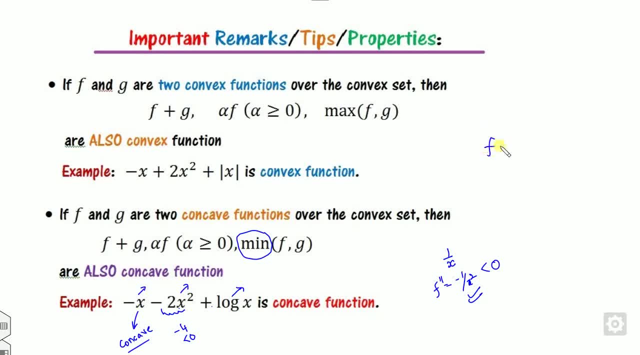 concave. So sum of the concave function is a concave function. Similarly, if I just take function as say 1, is the log x. second function is my say g as square root of 1 minus x square, and what is the minimum of f and g? So since log of x is a concave function, 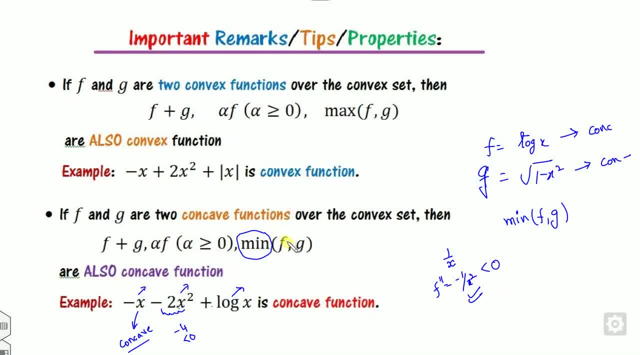 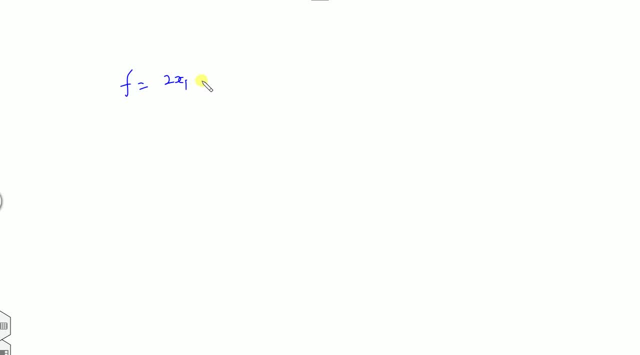 square root of 1 minus x square is a concave function and since both are the concave, so the minimum of them is also be the concave function. Similarly, if I just take the function as like, say this one: 2x1 plus 5x2 minus, 2x1, square minus x1, x2 plus. or you can say again: 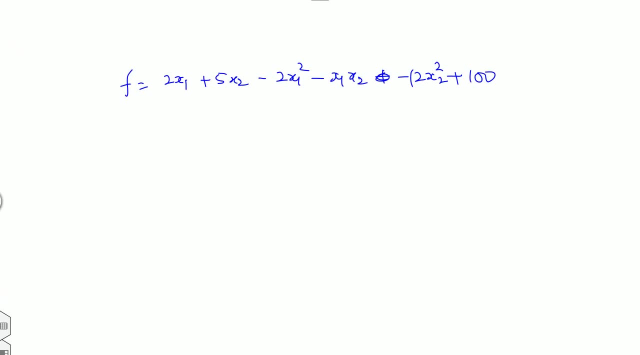 minus of the 2x2 square, that 12x2 plus 100 is there. Now you can check whether it is a concave or convex. First method is: you can draw the Hessian matrix and you can check Otherwise. this is a linear function. Linear is a convex as well as concave, both. 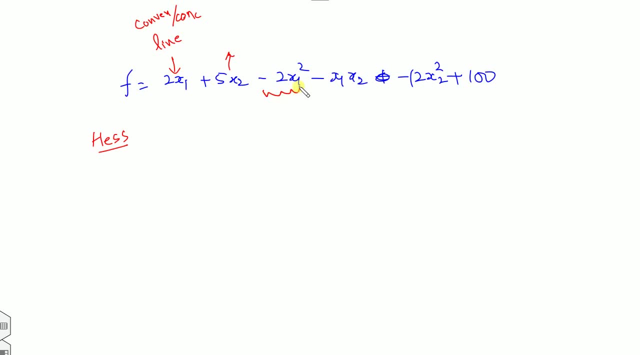 Again, it is a concave function. So this is a concave function. So this is a concave function, So this is a linear function. So convex and concave, both Minus of the 2x square. So 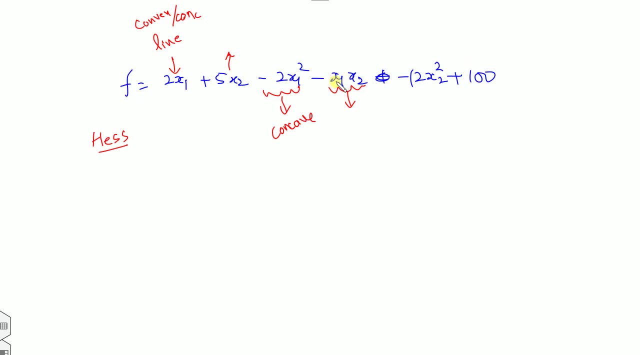 it is always be a concave. Look at that again. If you take the second derivative, this is a 0.. So it is a convex. Look at minus of the 12x square: It is always be a concave. 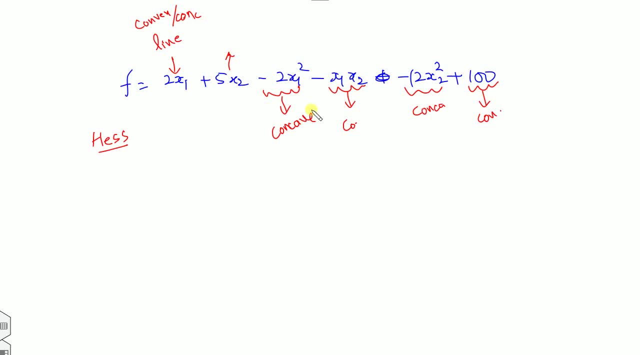 Every constant function is a convex and concave, So it is a concave. So, since some of the convex and concave function is a convex and concave, So this means this is a concave function. Look at that, If I just take the x1 square plus x2 square is a convex, or? 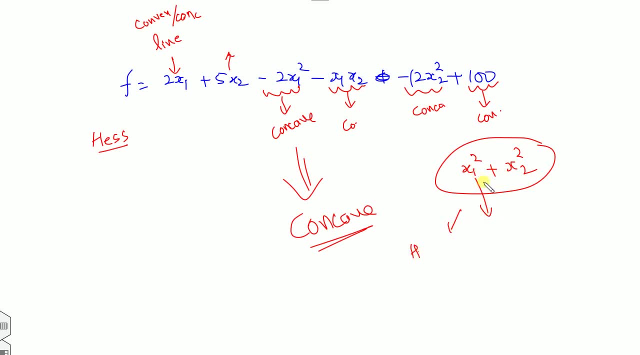 concave. Either you can draw the Hessian matrix, Else what is the x1 square? This is a concave convex function because it is a u-shape, or the second derivative is greater than 0.. What is the x2 square? It is again a convex function. So it is a convex function, If I just take another. 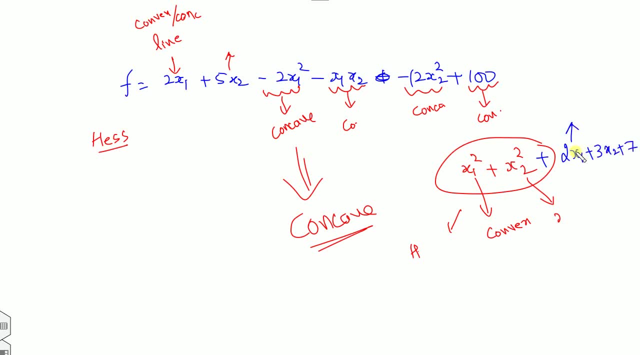 function here, like, say, 3x2 plus 7.. This is a linear function. So every linear function is a convex also. Every linear function is a convex also. Every constant function is a convex also. So again, this is a convex function. So this is the way you can check. 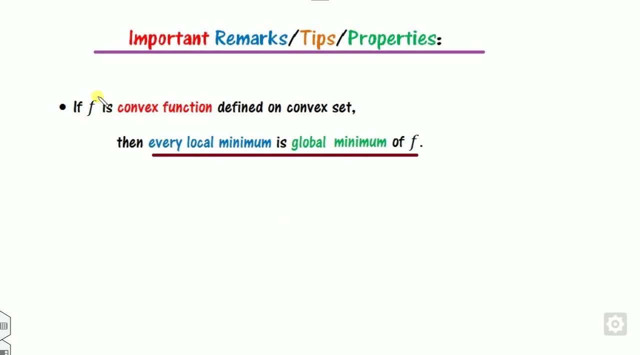 Whether the convex or concave, in a very easy manner. Another point is that if f is my convex function, then every local minimum is a global minimum. So this is one of the most important concept that we will see in our convex optimization problem. Another point in remark is that if f of x 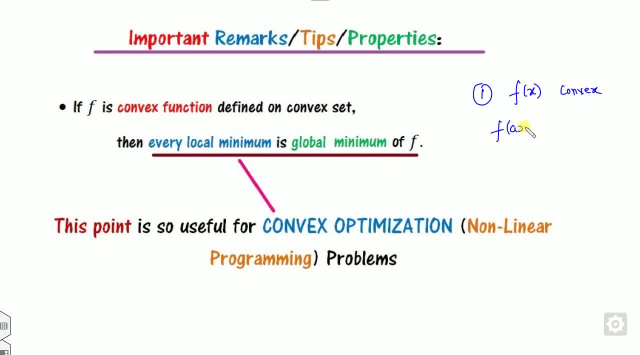 is my convex function, then f of ax plus b is also a convex function, provided a and b are my constant. For example, if I take a convex function, then f of x is my convex function. So let me say, mod of 2x plus 3 is a convex or not. Look at that. mod x is always be a convex function. 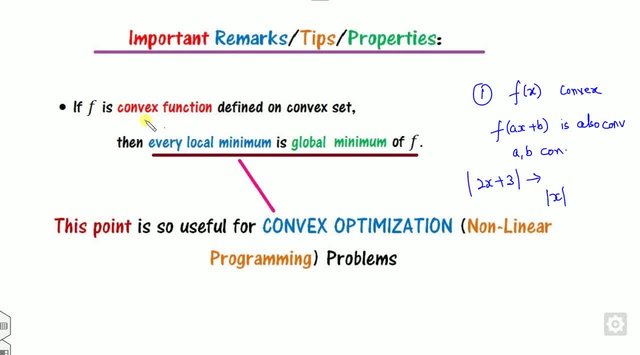 So 2x plus 3 is also a convex function. Now, since a convex, the important property of the convex function is: every local is a global, And this is most useful when we study the convex optimization technique. And that is our next lecture. So before understanding this next, 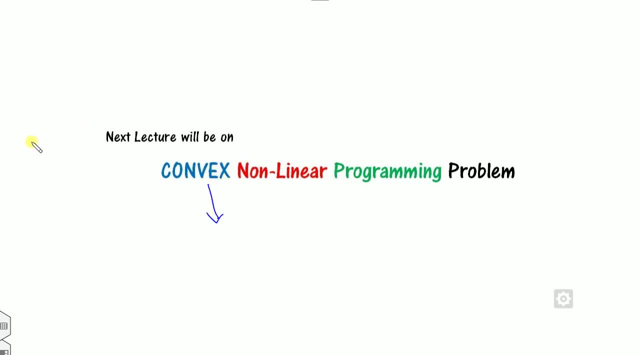 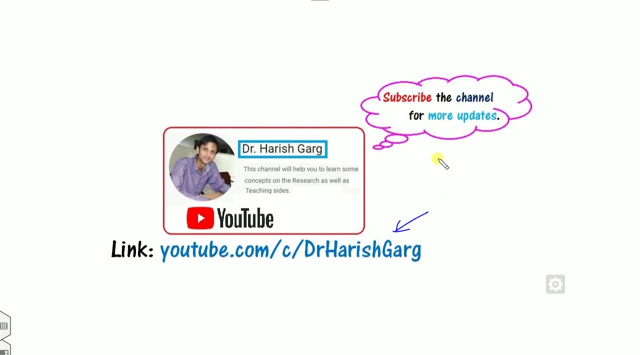 lecture. you have to understand how you can check whether the function is convex or not. So this is the so far we have discussed here. If you feel any doubt, you can ask me. Else, you can simply follow this link. You can share the video to the other friends also. Till then, best of luck students.